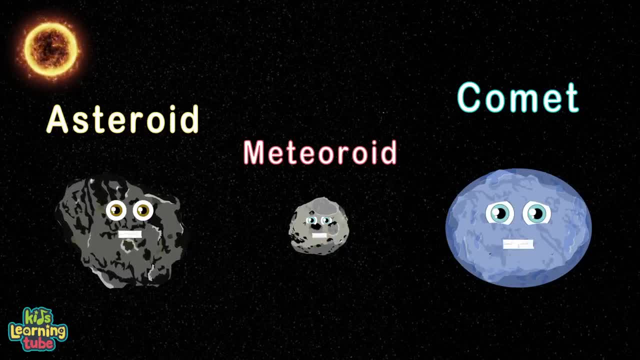 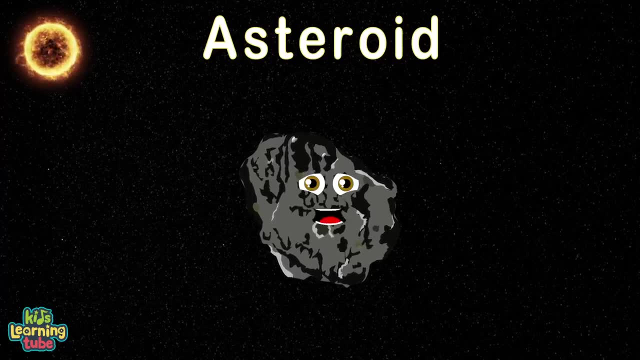 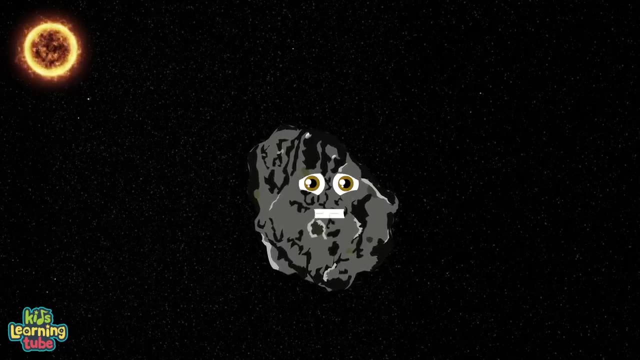 We're all part of this universe. Let's give these space rocks their turn. I'm an asteroid, also called a minor planet, to some, A rocky, airless remnant left over from our solar system's formation. You can find a lot of asteroids orbiting our sun. 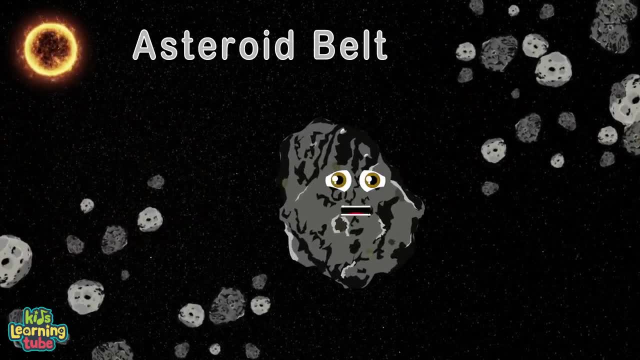 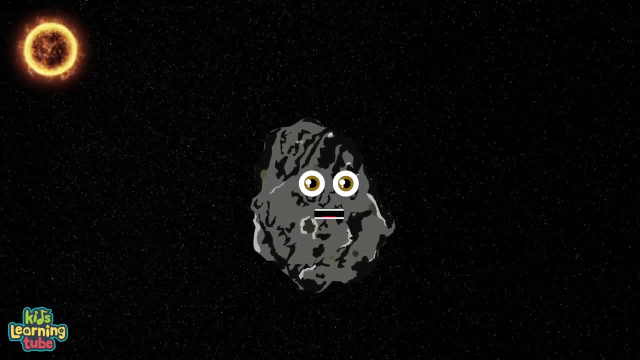 Between Mars and Jupiter within the asteroid belt I run. I can range in size from about 329 miles down to 33 feet small. I've been here for a while. I'm made up of different kinds of rocks and some have clays in them. 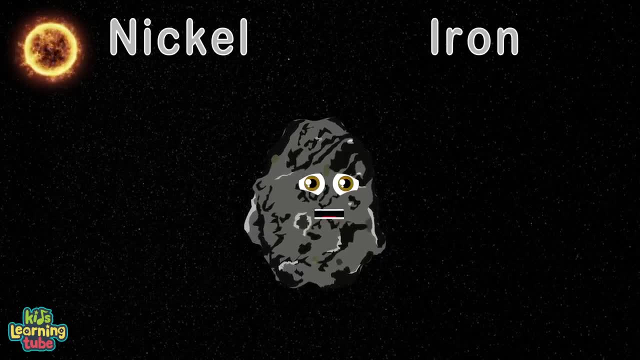 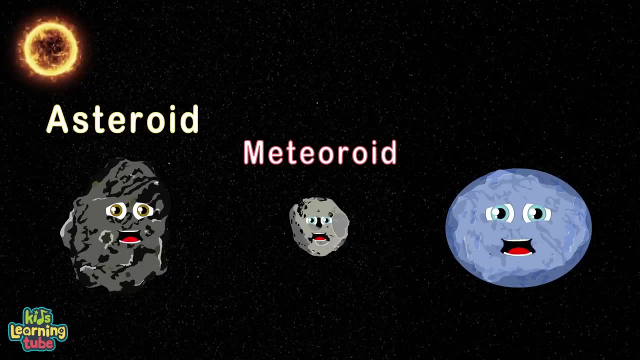 Such as nickel and iron, found in frying pans or kettles. Here's the difference between these space rocks that you will see, Asteroid, Meteoroid and Comets and some. what stages between These different celestial bodies are important to learn. 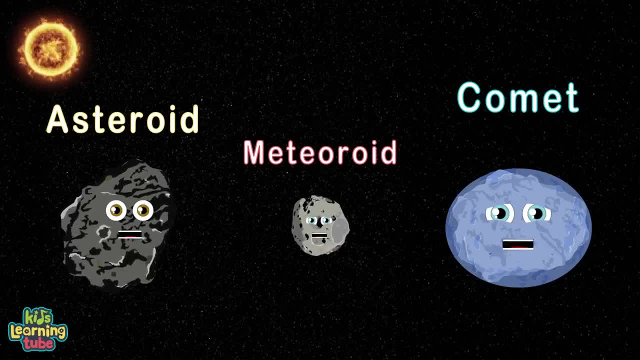 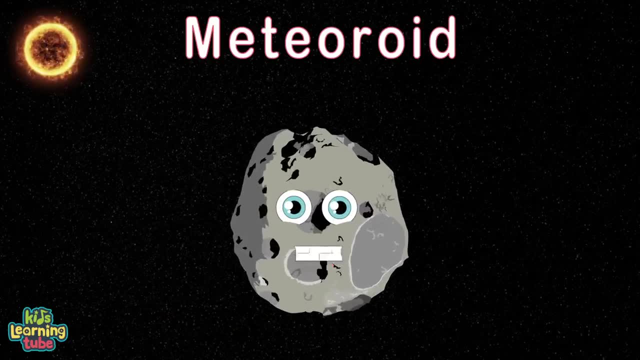 We're all part of this universe. Let's give these space rocks their turn. I'm a Meteoroid. I'm smaller than an asteroid. you see, My size can range from a grain of dust to a small asteroid. Yeah, that is me. 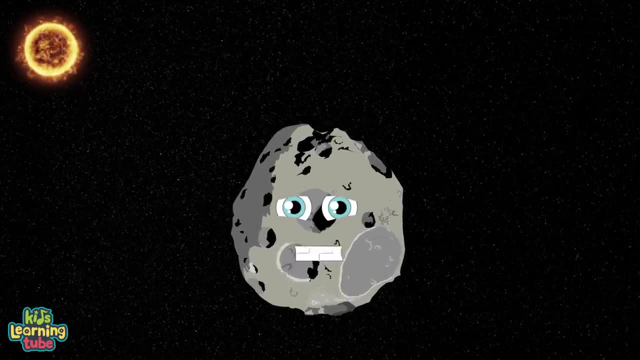 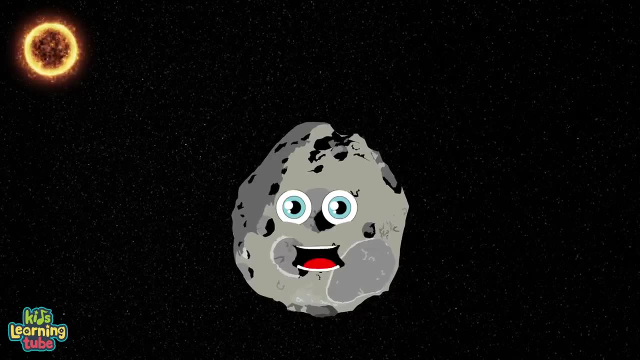 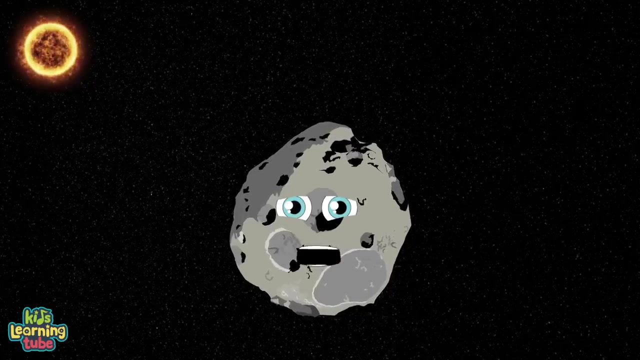 I orbit the sun. I'm made of minerals called silicates, Which is silicone and oxygen. I'm glad that you're learning this. I'm also made of heavier metals like nickel and iron. Let's go explore a little more about what other names I can become. 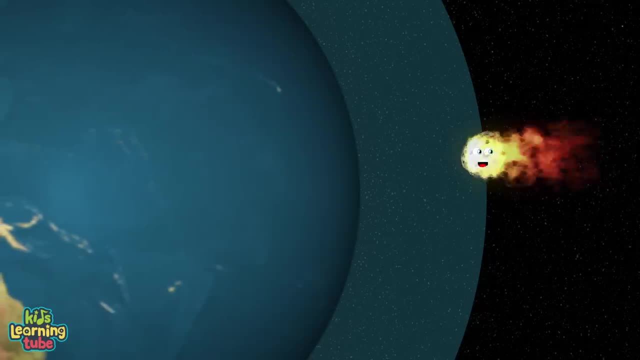 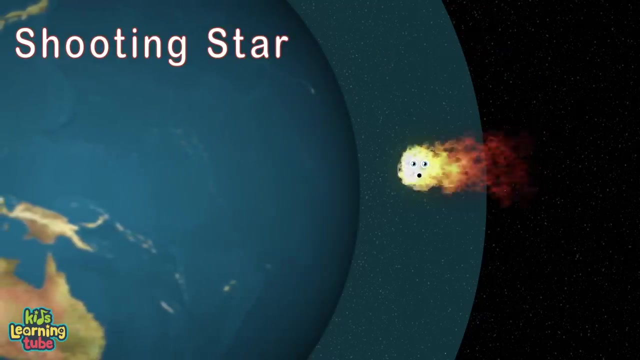 If I enter Earth's atmosphere, you'll see a bright tail of light. If this happens and I vaporize, I'm called a meteor. that's right. Some call me a shooting or falling meteor. I'm only called a meteor if I burn up completely. 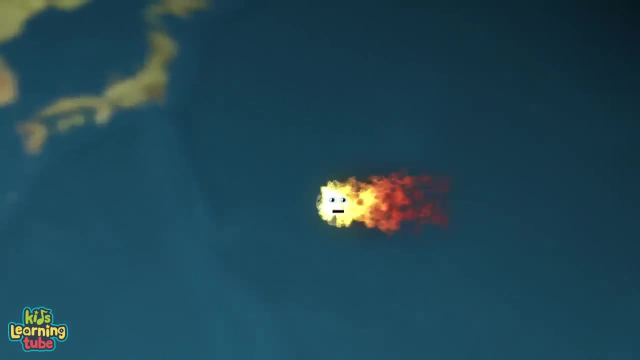 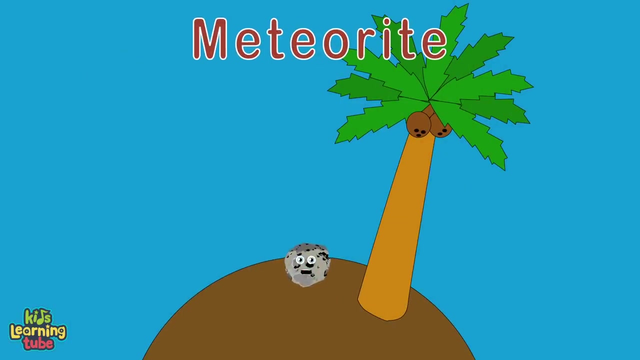 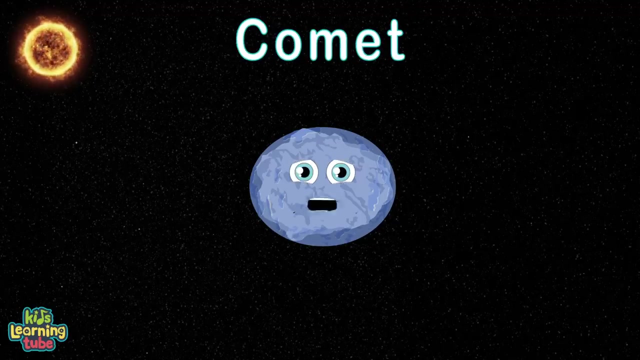 It's bizarre, But if I make it through the atmosphere and reach the Earth's surface, My name changes to meteorite. It is important to learn this. I'm a comet, which is dust mixed with frozen gas. When fully frozen, I'm about the size of a small town. 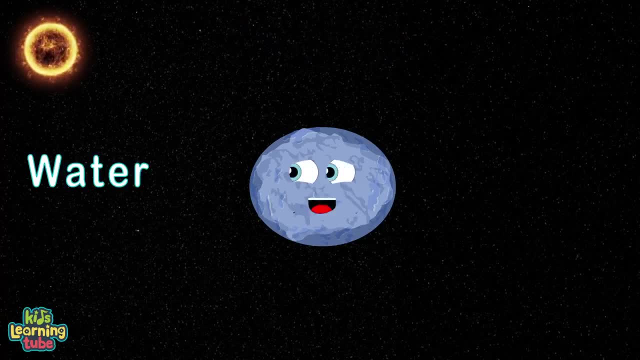 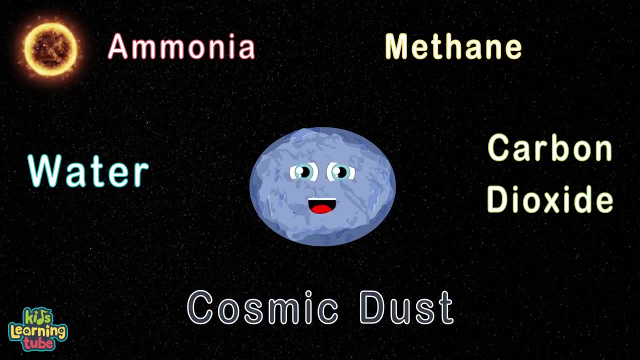 Through space I do pass. I'm made of ices like water, carbon dioxide, ammonia and methane, Mixed with cosmic dust from our solar system. when it begins, When I get close to the sun, I heat up and spew dust and gas.